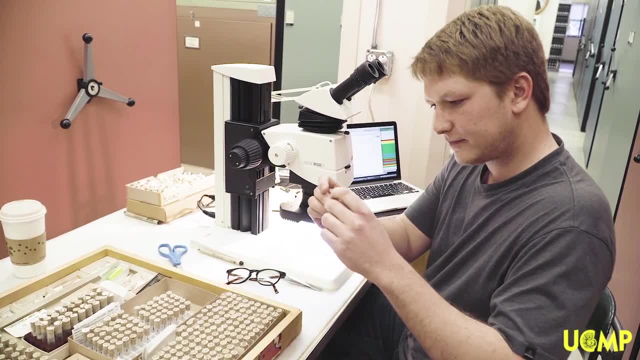 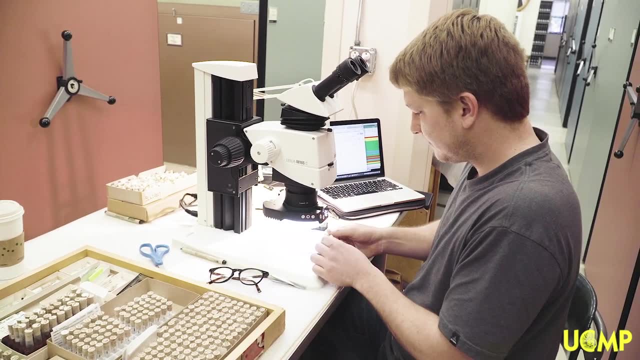 material of multi-tuberculate specimens from a locality that's coeval with this Judith River material. It's the two medicine formation and we have some complete skeletons and skulls and dentitions of multi-tuberculate that I'll be describing there. So my reasoning for 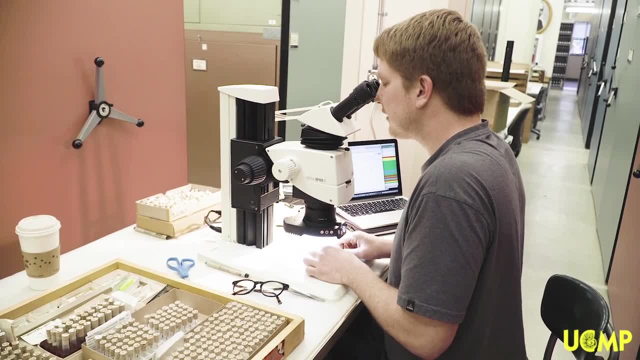 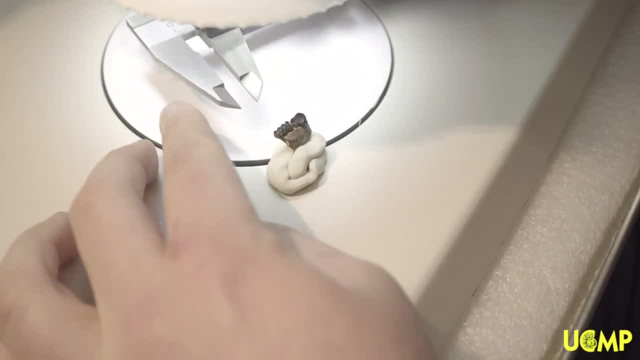 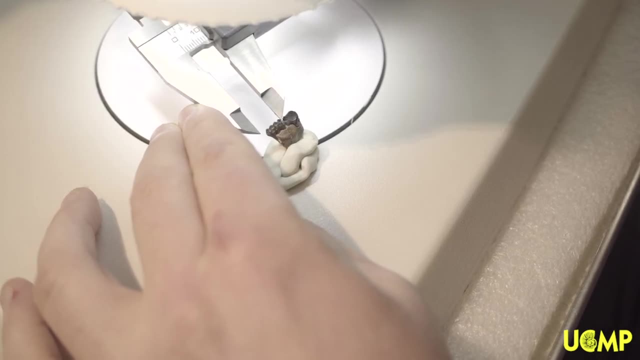 coming here was both to compare the Judith material to those materials and then also to take different linear measurements on different aspects of the teeth and note certain characteristics of their morphology to help a broader project which is aiming to understand the relationships between some of the earliest groups of the multi-tuberculates that later in the Cretaceous 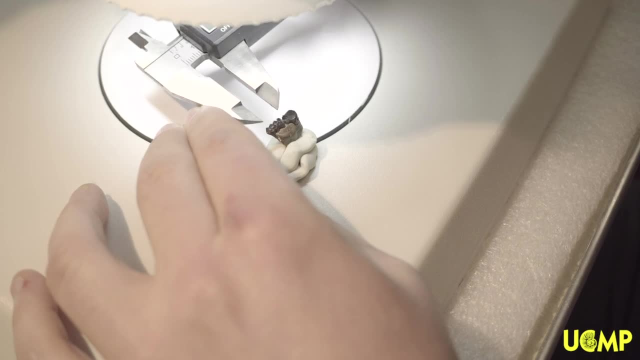 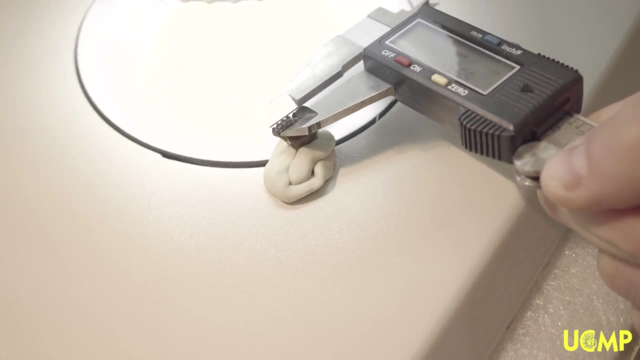 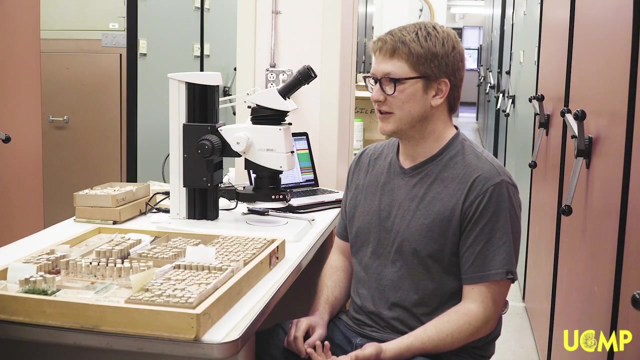 go on to be the most dominant, both in number of species and as far as kind of ecological diversity, in the later Cretaceous And into the early Paleogene as well. So basically measuring teeth and taking lots of notes and pictures as well. So basically, multi-tuberculate mammals- they're the longest lived order of. 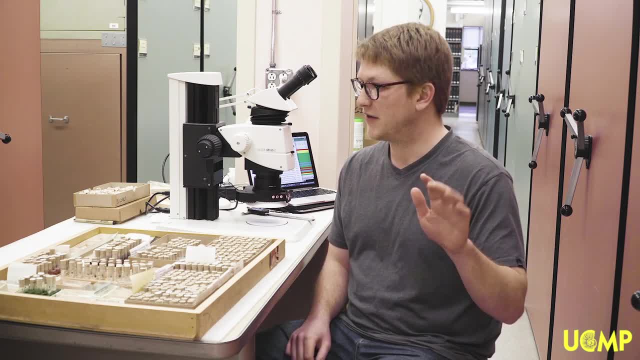 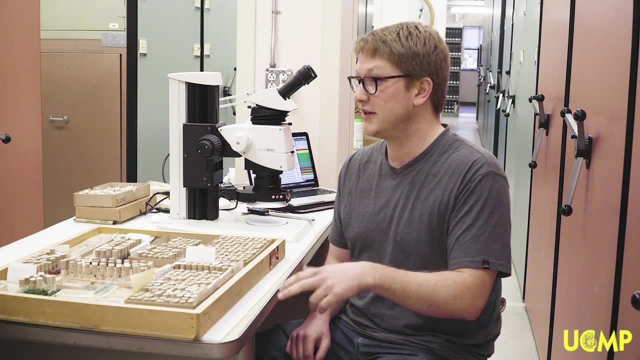 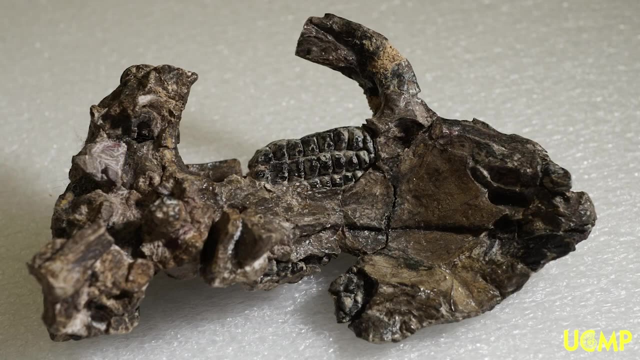 mammals. They show up in the fossil record of about the middle Jurassic and they persist until the end of the Eocene, So a span of about 166 to 35 million years. And what they're? they're characterized by these really funky teeth, So they have molars that have a bunch of 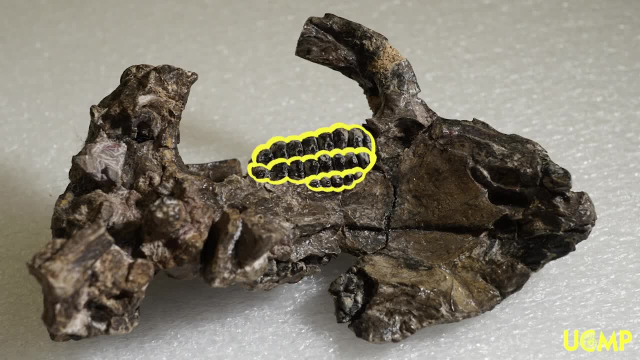 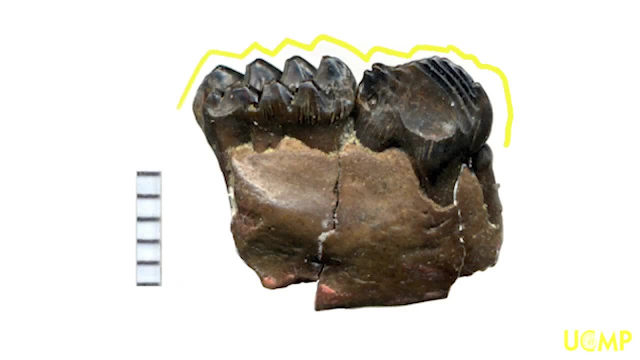 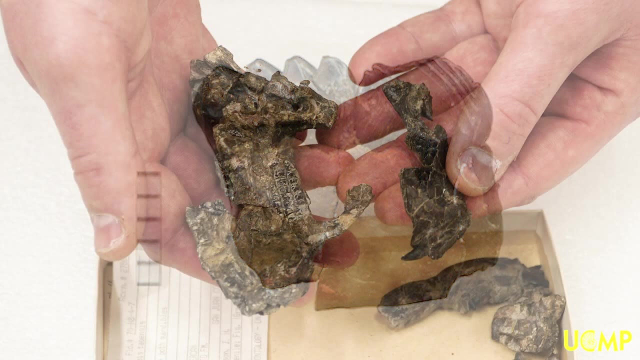 little bumps arranged in kind of longitudinal rows, and they have a big fourth premolar on their lower jaw that is shaped kind of like a buzzsaw. So multi-tuberculate literally means multiple tubercles. so many bumps. essentially They're an extinct lineage, So they were by far the most. 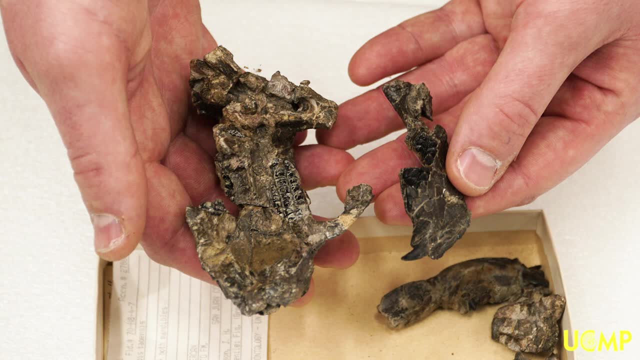 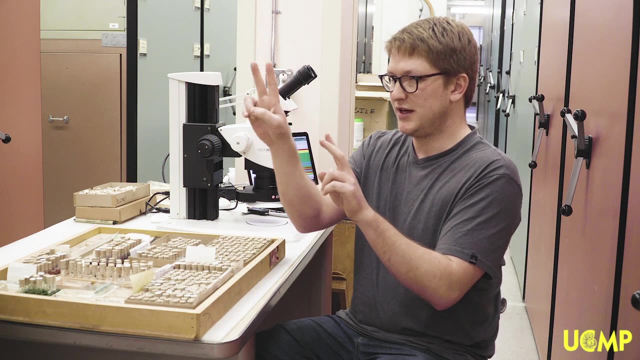 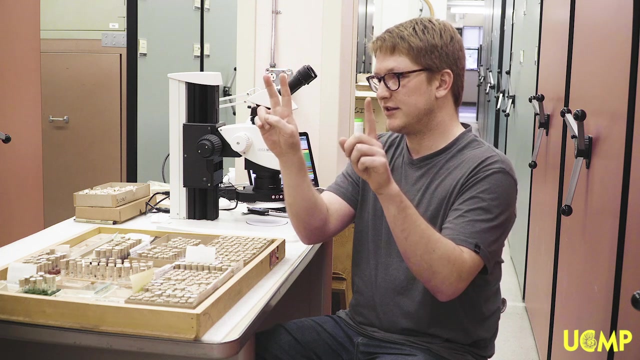 abundant and diverse group of mammals in the late Cretaceous, but they're now extinct. Their closest relatives is often debated, but and so multi-tuberculates are essentially sitting phylogenetically between um, um, um, um, placentals and marsupials, which we call Therian mammals, and the monotremes, So they're kind of 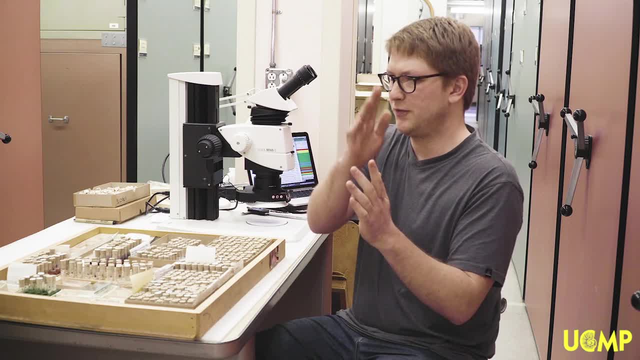 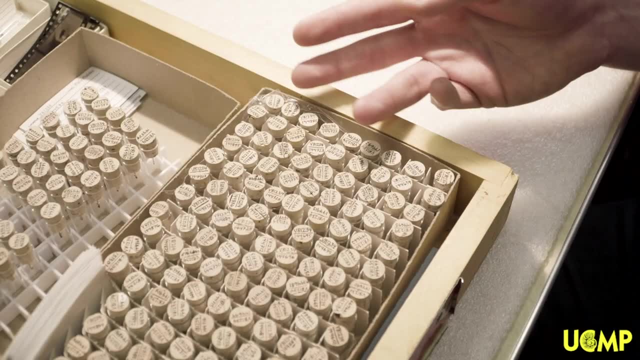 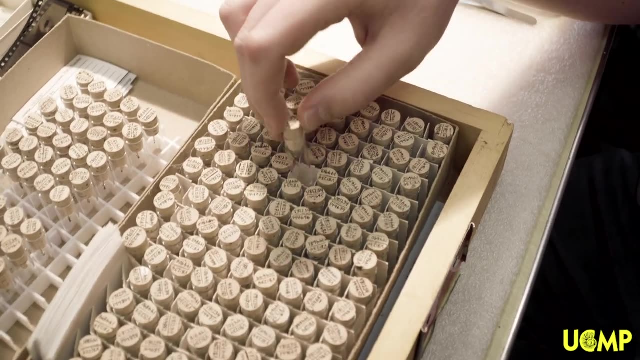 in between there And there's a bunch of other Mesozoic mammal groups with kind of fall on that gradient between those two major living groups. So what you're looking at when you see these seas of corks is basically they're the backsides of pinned teeth. So Mesozoic mammals as a rule.